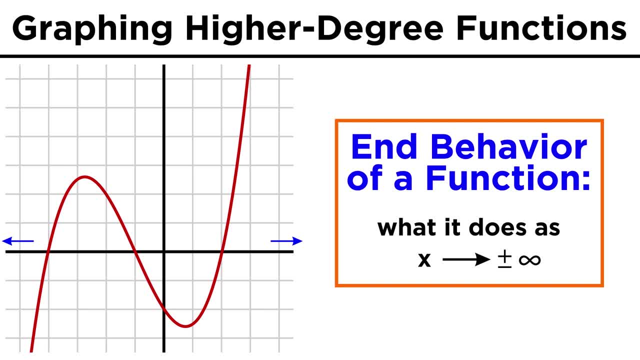 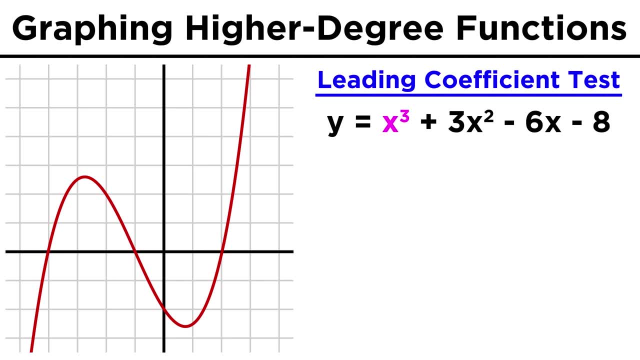 to figure out what the end behavior of a function will be. We can do this by using something called the leading coefficient test. We look at the leading term in a polynomial, or the term with the largest exponent, and we look at its exponent and its denominator. 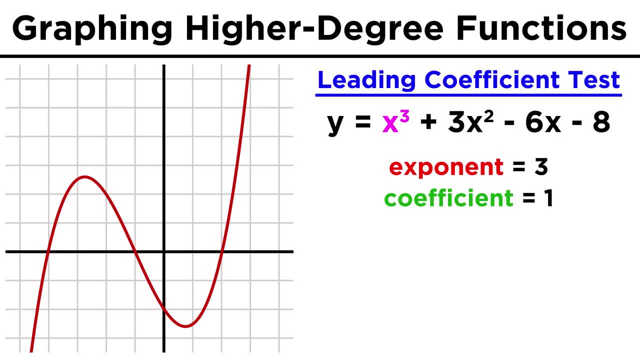 Depending on whether the exponent is even or odd and whether the coefficient is positive or negative. we know what the end behavior will be. If the exponent is odd, such as with a cubic function or one that starts with x to the fifth, x to the seventh, and so forth. if the leading coefficient is positive, the function 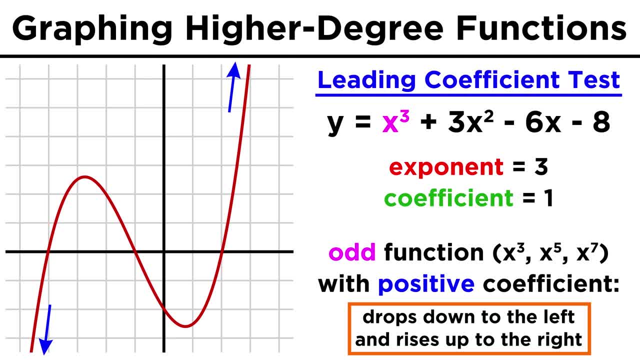 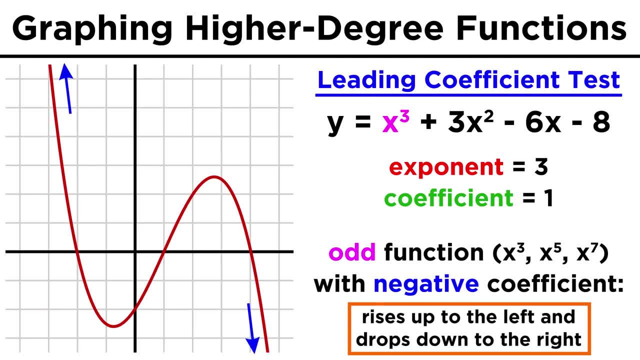 will fall downwards to the left and rise upwards to the right. If the leading coefficient is negative, the function will rise upwards to the left and fall downwards to the right. We don't yet know what will happen in the middle, but this end behavior is a great start. 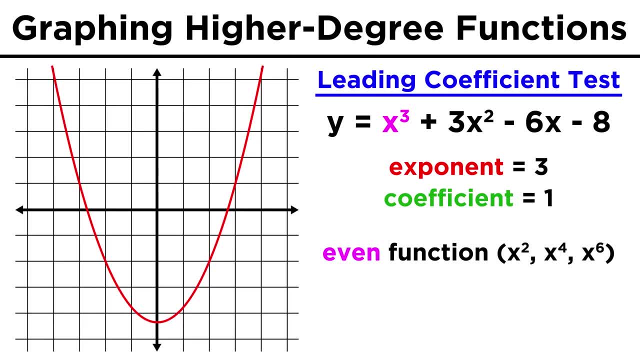 in terms of sketching the function, Then if the exponent is even such as with quadratic or quartic functions, or ones beginning with x to the sixth, x to the eighth, and so on, if the leading coefficient is positive, the function will rise upwards on both sides. 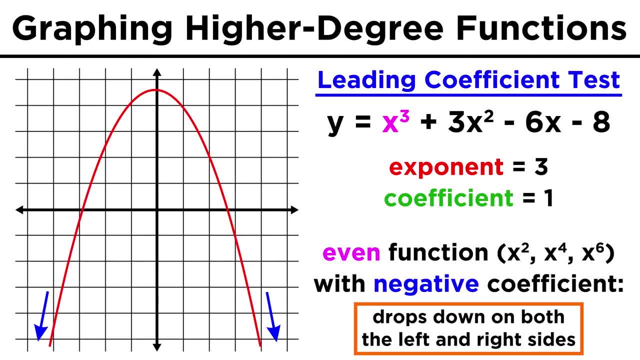 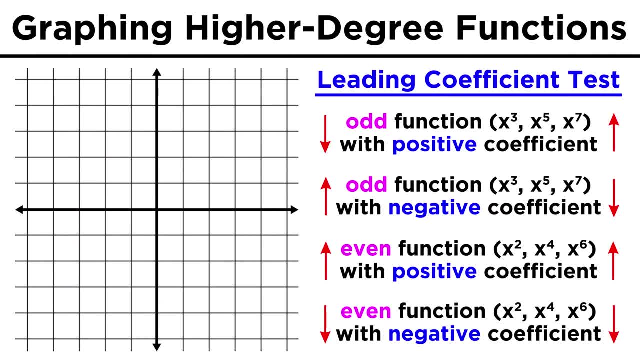 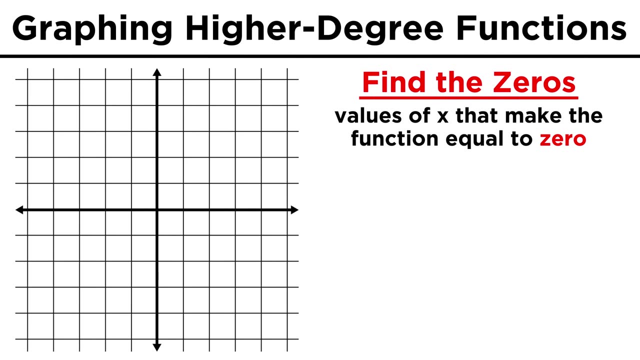 If the leading coefficient is negative, the function will fall downwards on both sides. So those are the four possibilities in terms of the end behavior of higher degree polynomials. Now that we have the end behavior, the next thing to do is to find the zeros of the function. 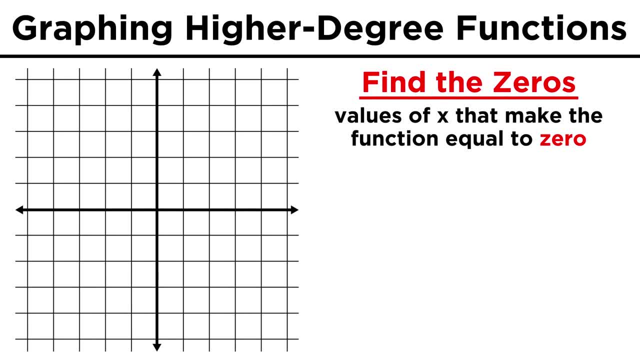 These will be the values of x that make the function equal to zero, which can be understood graphically as x-intercepts, because these are points where y equals zero. To get these, we set the function equal to zero and solve for x. 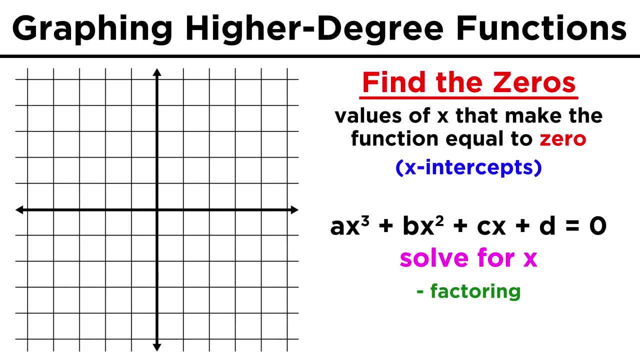 This can be very tricky, but sometimes a little factoring will do it. Other times we have to use the rational roots test in conjunction with synthetic division to find out what the zeros are. We learned this technique earlier in the series, so it would be a very good idea to check out. 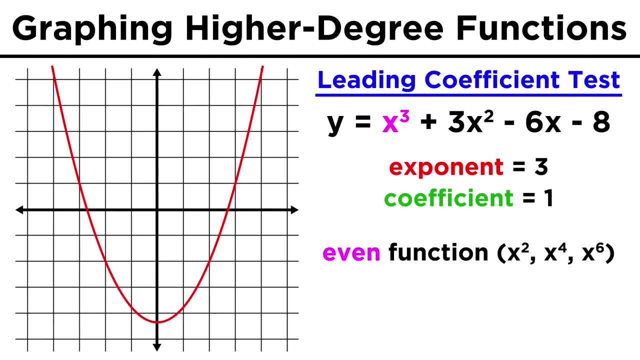 in terms of sketching the function, Then if the exponent is even such as with quadratic or quartic functions, or ones beginning with x to the sixth, x to the eighth, and so on, if the leading coefficient is positive, the function will rise upwards on both sides. 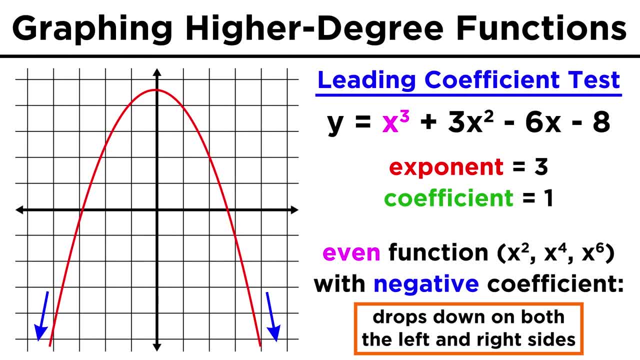 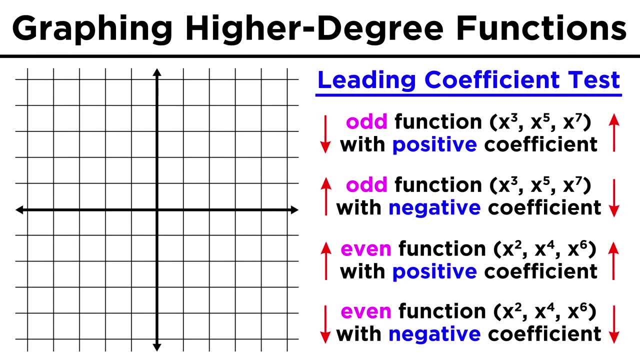 If the leading coefficient is negative, the function will rise upwards to the left and fall downwards on both sides. If the leading coefficient is negative, the function will fall downwards on both sides. So those are the four possibilities in terms of the end behavior of higher degree polynomials. 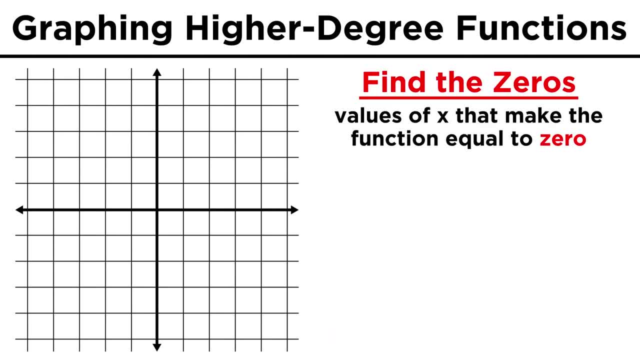 Now that we have the end behavior, the next thing to do is to find the zeros of the function. These will be the values of x that make the function equal to zero, which can be understood graphically as x-intercepts, because these are points where y equals zero. 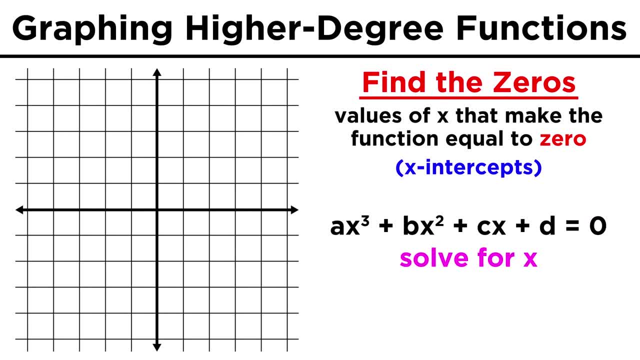 To get these, we set the function equal to zero and solve for x. This can be very tricky, but sometimes a little factoring will do it. Other times we have to use the rational roots test in conjunction with synthetic division to find out what the zeros are. 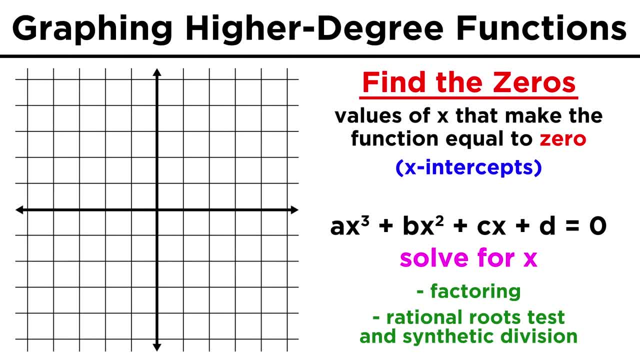 We learned this technique earlier in the series, so it would be a very good idea to check out these tutorials right now If you need to learn how to graph higher degree polynomials. To see what to do once we find the zeros, take something like x cubed plus three x squared. 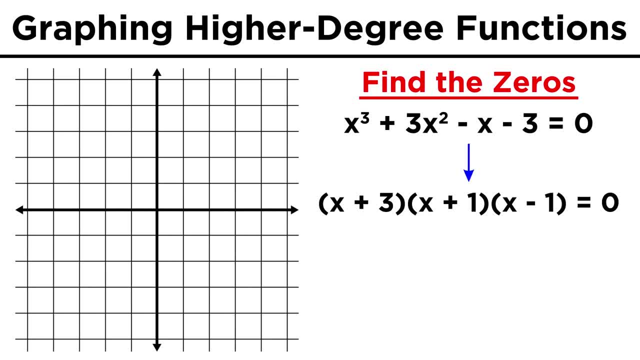 minus x minus three equals zero. If we can factor this or perform synthetic division, we can eventually express this as x plus three times x plus one times x minus one. That means that the x-intercepts are negative three, negative one and one. 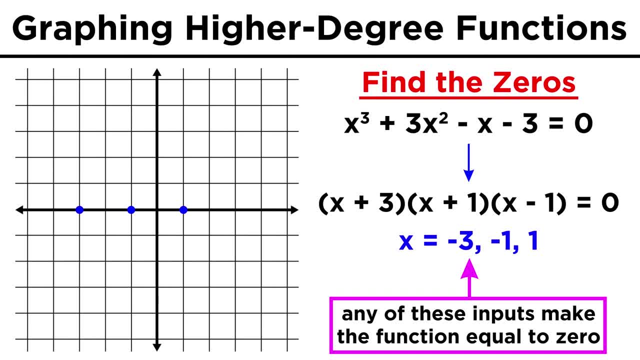 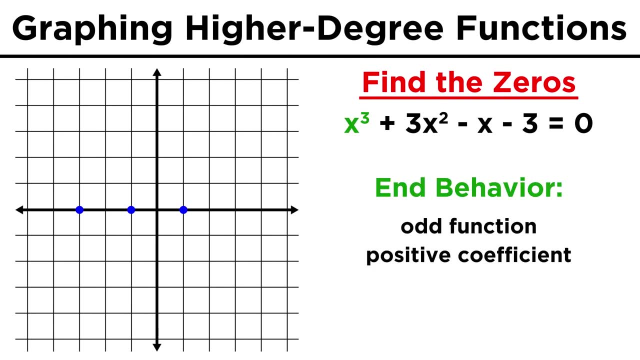 Since any of these values will make one term equal to zero and thus the whole function will be equal to zero, since anything times zero is zero. So we can plot these three points for the function right on the x-axis. Then we can get the end behavior by noticing that the leading term has an odd exponent. 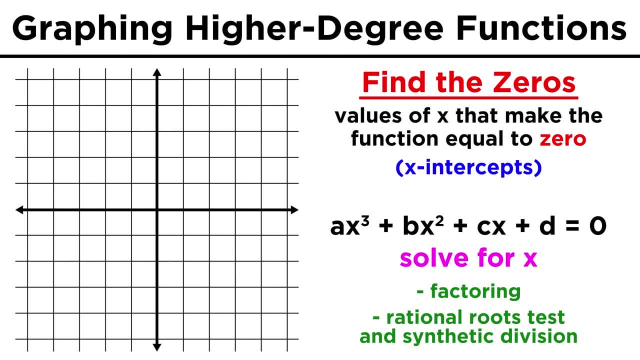 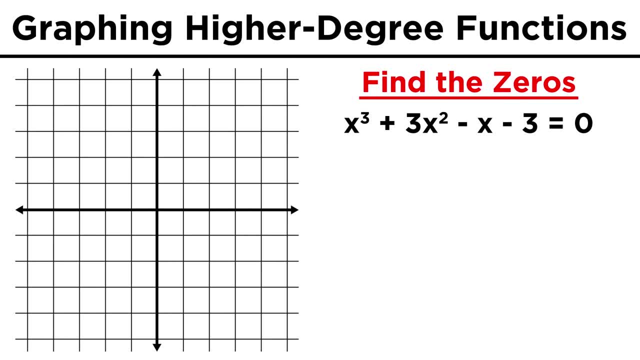 these tutorials right now If you need to learn how to graph higher degree polynomials To see what to do once we find the zeros. take something like x cubed plus three, x squared minus x minus three equals zero. If we can factor this or perform synthetic division, we can eventually express this as: 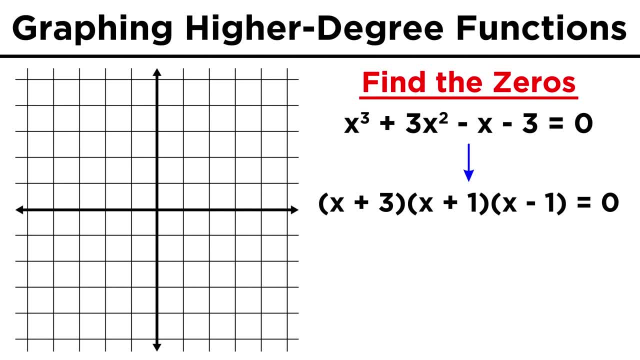 x plus three times x plus one times x minus one. That means that the x-intercepts are negative, three negative one and one, Since any of these values will make one term equal to zero and thus the whole function will be equal to zero, since anything times zero is zero. 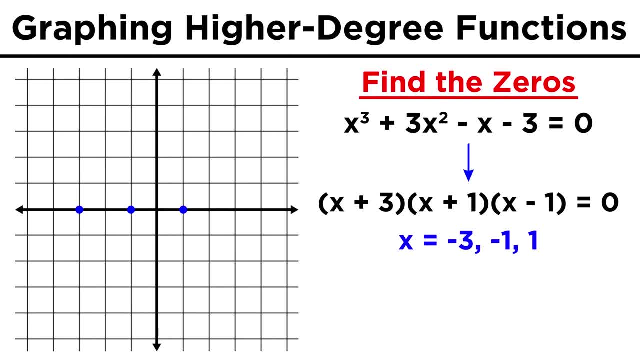 So we can plot these three points for the function right on the x-axis. Then we can get the end behavior by noticing that the leading term has an odd exponent and a positive coefficient of one, meaning that the function falls to the left and rises. 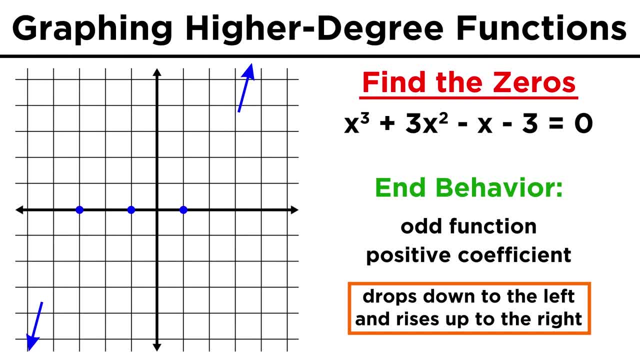 to the right. This is already enough information to sketch this function, because going left to right, it must rise up from negative infinity, cross the x-axis at this point, curve back down and cross again here, curve up and cross one more time and then rise up towards positive. 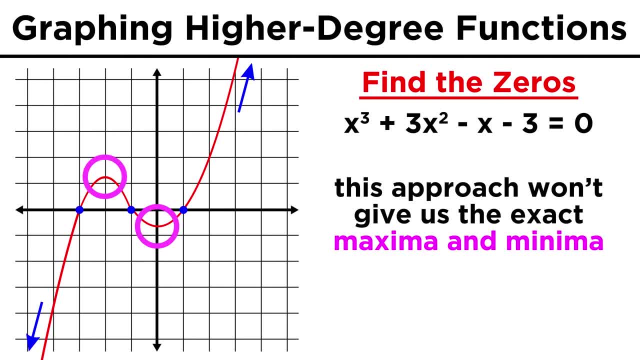 infinity. It's true that we aren't getting the exact maxima and minima when using such an approach. That would require calculus, So this isn't an issue. This is an exact representation, But the function must indeed look roughly like this, and sometimes that's all we need. 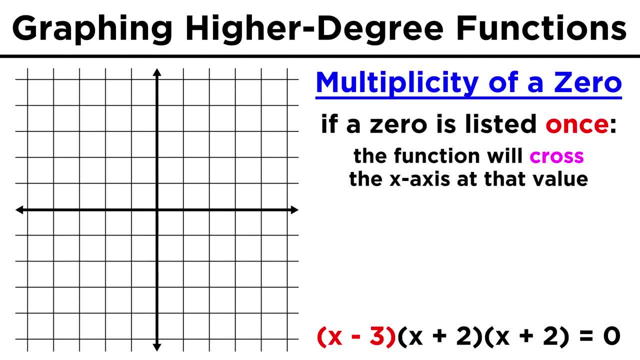 to know. We must point out one other thing at this time. If a zero is listed precisely once when a function is expressed as its factors, the function will cross the x-axis at that value. But if a zero is listed twice, then the function will touch the x-axis at that value and then 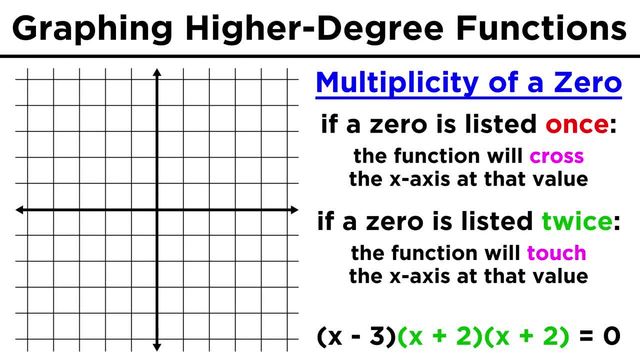 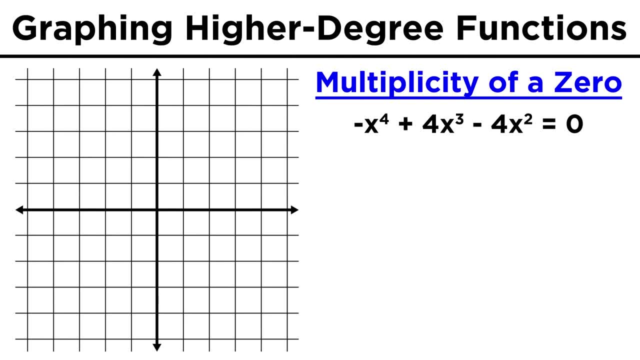 curve back in line. This means that if a zero is listed twice, then the function will cross the x-axis at that value and then curve back in the direction it came from. For example, take negative x to the fourth, plus four x cubed, minus four x squared. 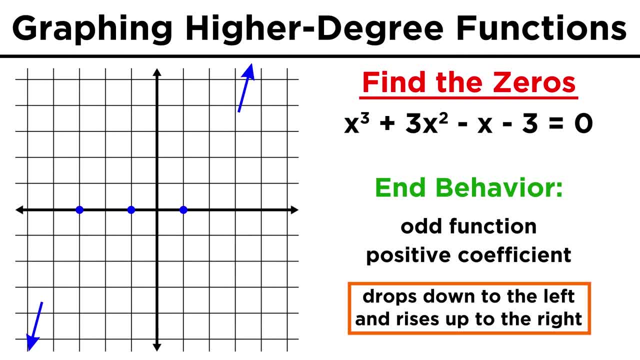 and a positive coefficient of one, meaning that the function falls to the left and rises to the right. This is already enough information to sketch this function because, going left to right, it must rise up from negative infinity, cross the x-axis at this point, curve back down. 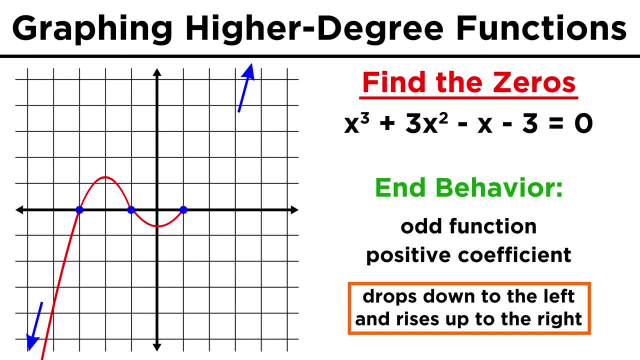 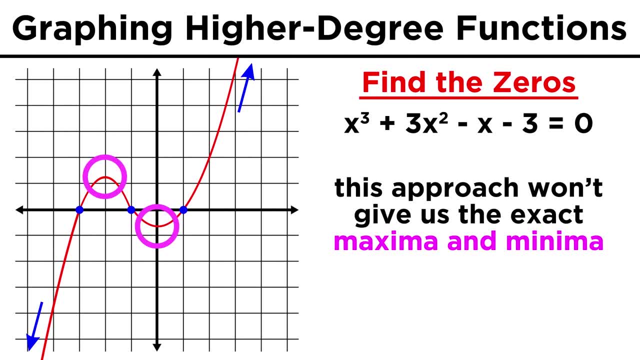 and cross again here, curve up and cross one more time and then rise up towards positive infinity. It's true that we aren't getting the exact maxima and minima when using such an approach. That would require calculus. So this isn't an exact representation, but the function must indeed look roughly like. 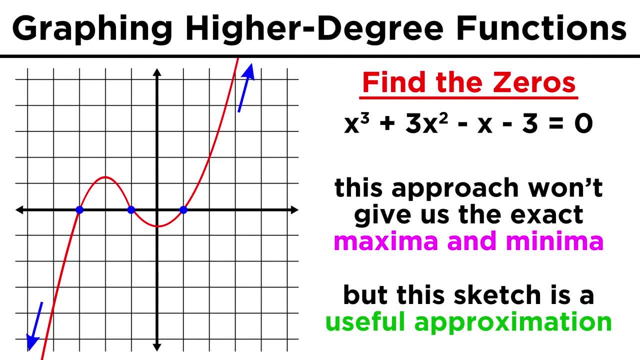 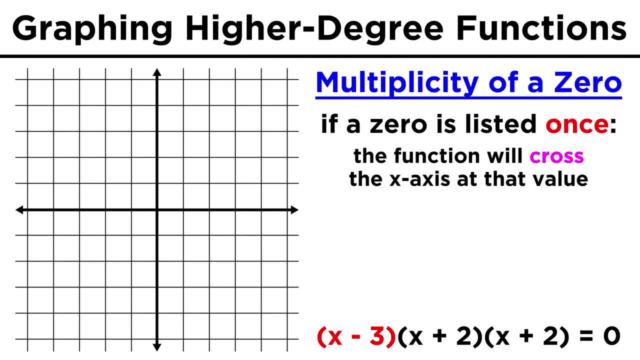 this, and sometimes that's all we need to know. We must point out one other thing at this time: If a zero is listed precisely once when a function is expressed as its factors, the function will cross the x-axis at that value. But if a zero is listed twice, then the function will touch the x-axis at that value and then 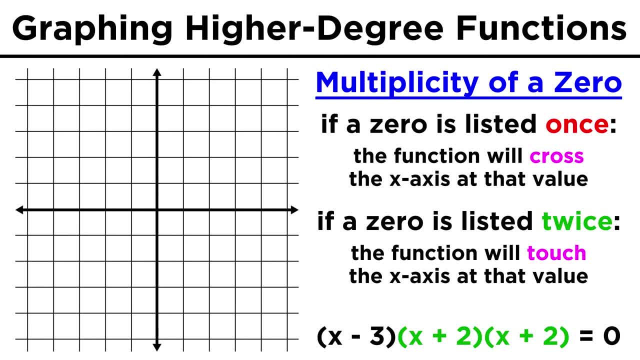 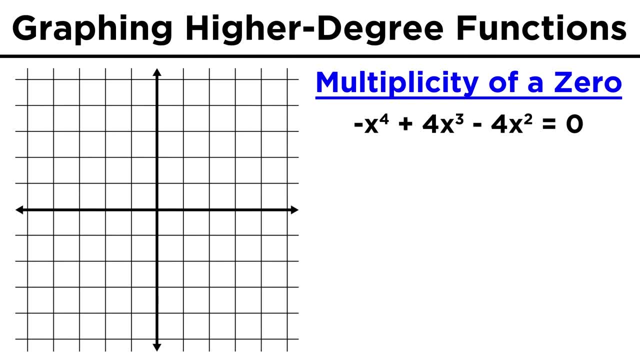 curve back in the direction it came from. For example, take negative x to the fourth plus four x cubed, minus four x squared. We could do synthetic division or just recognize that we can factor out negative x squared. Then this perfect square can be expressed as x minus two quantity squared. 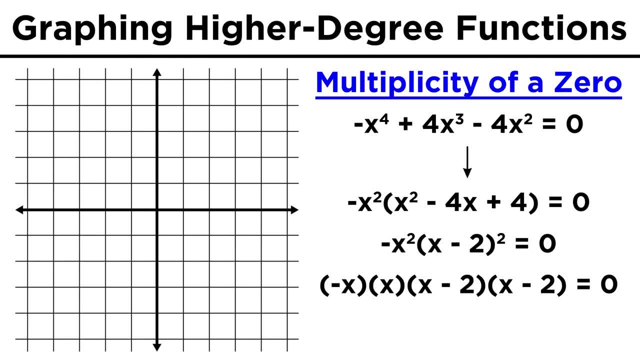 We can either leave it like this or understand that this also means negative x times x times x minus two. This means that zero is one of the zeros, but it is a zero twice. Positive two is another zero, but it is a zero twice. 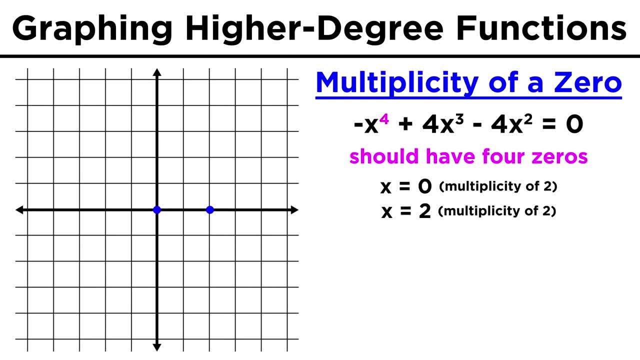 This makes sense because a quartic function should have four zeros and each of these just has a multiplicity of two, Finding the n behavior. the leading exponent is even and the coefficient is negative, so this should fall twice. It should not fall towards negative infinity on either side. 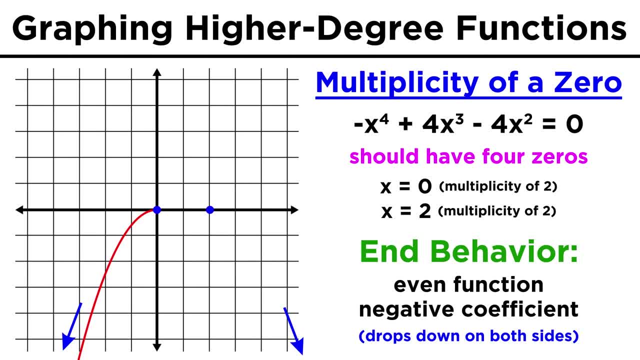 Given what we just said about zeros that occur twice, the function must rise up from the left, touch the x-axis at x equals zero, but then curve back down. curve back up to touch the x-axis again at x equals two, and then fall back down towards negative infinity. 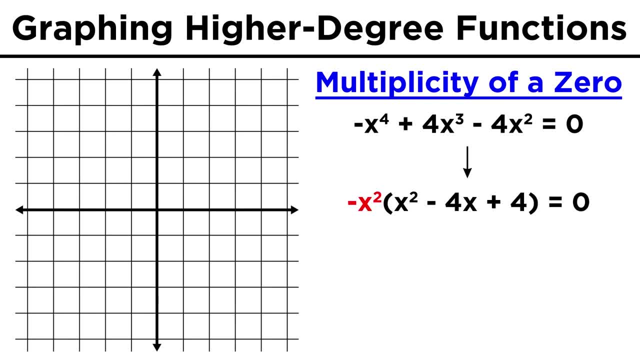 We could do synthetic division or just recognize that we can factor out negative x squared. Then this perfect square can be expressed as x minus two quantity squared. We can either leave it like this or understand that this also means negative x times, x times. 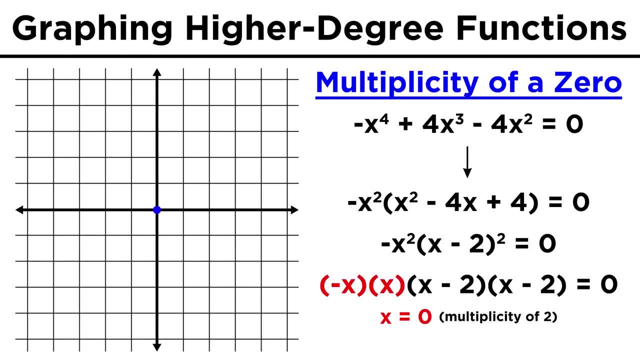 x minus two times x minus two. This means that zero is one of the zeros, but it is a zero twice. Positive two is another zero, but it is a zero twice. This makes sense because a quartic function should have four zeros and each of these. 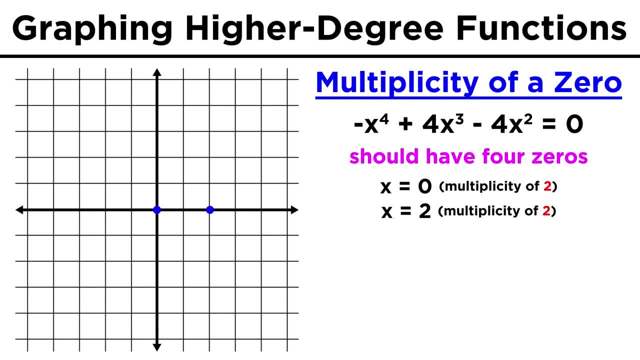 just has a multiplicity of two Finding the end behavior. the leading exponent is even and the coefficient is negative, so this should fall towards negative x, Negative infinity on either side. Given what we just said about zeros that occur twice, the function must rise up from the 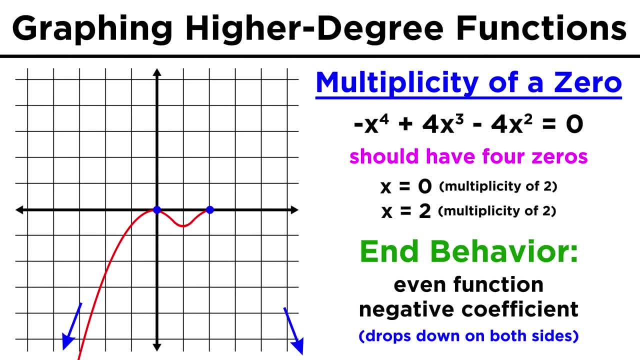 left. touch the x-axis at x equals zero, but then curve back down, curve back up to touch the x-axis again at x equals two, and then fall back down towards negative infinity Again. this isn't flawlessly precise, but for many purposes this is good enough. 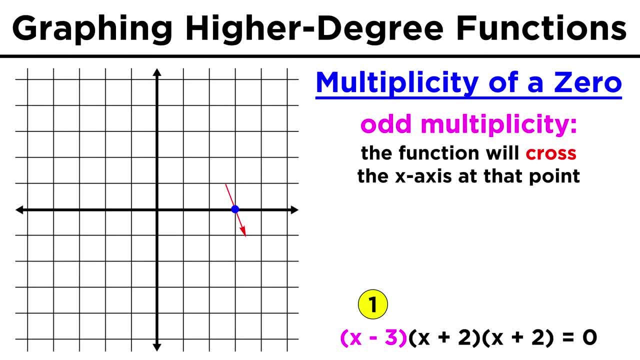 So what we can say is that if a zero has an odd multiplicity, like one or sometimes three or greater, the function will cross the x-axis. at that point, If a zero has an even multiplicity- usually two, but sometimes more- the function will. 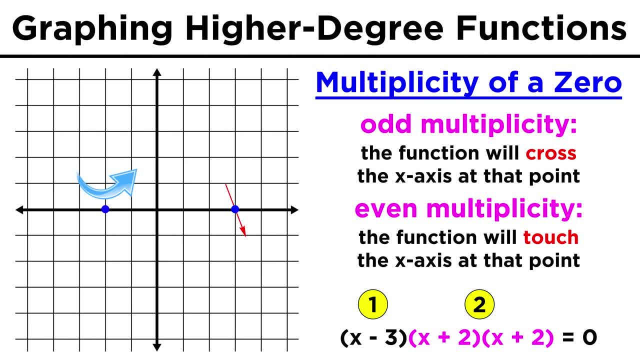 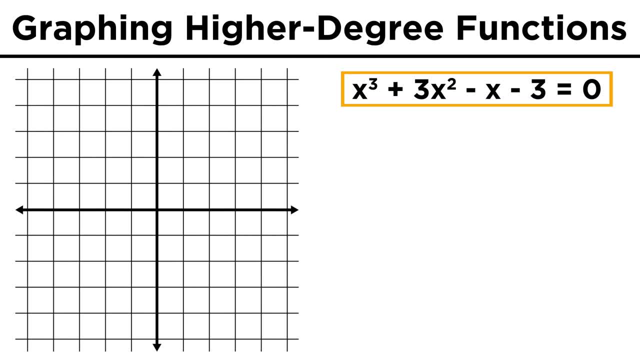 touch the x-axis at that point and then turn around. So now we have a solid strategy for graphing higher degree polynomials. Start with the leading coefficient two. Start with the leading coefficient test to find the end behavior of the function. Then find the zeros of the function by whatever method necessary, whether factoring or the. 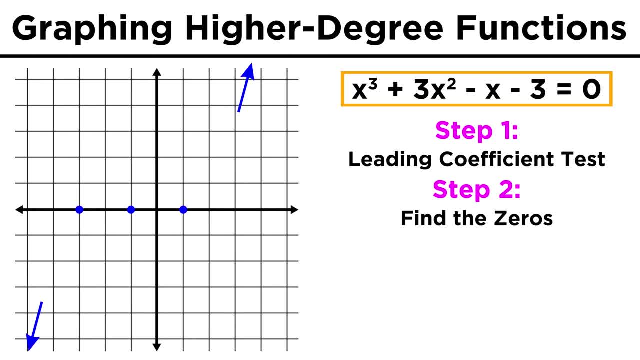 rational roots test and synthetic division, Then assess the multiplicity of each zero to find out whether the function will cross or just touch the x-axis at each zero. If we want one more additional point, we can easily get the y-intercept, which means that